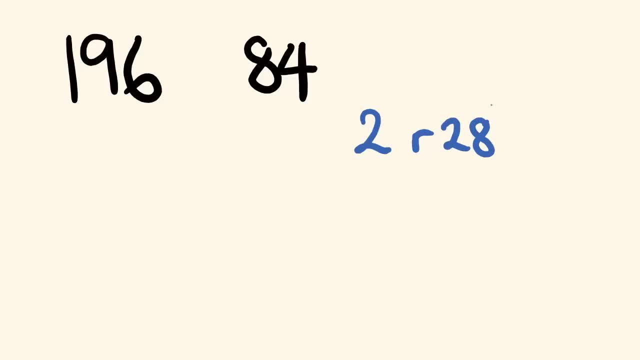 be worried about for the next step. We're going to move this remainder on to the next step. Okay, so 28,. we're moving on to this next step. The other part we move to the next step is the smallest of our numbers, the ones that we divided into one another. In this case it was the original. 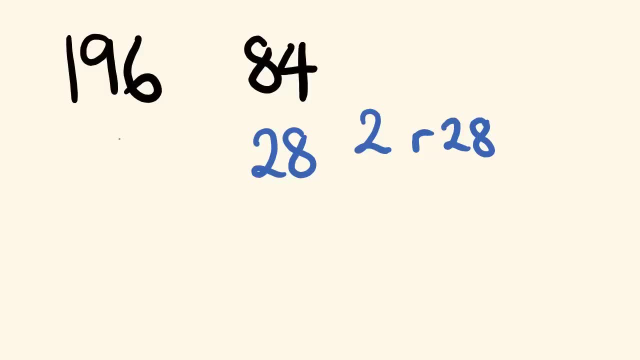 two numbers. We had 196, 84.. The smallest is 84. But if we were going on to the next, you know, another step and another step, we'd choose the smallest out of, say, these two. Okay, so what we? 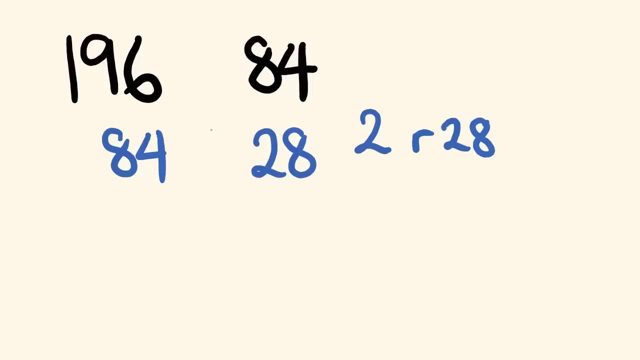 do? is we repeat this step? How many times is 28?? Go into 84.. Hey, it goes in three times. It goes in three times and there is no remainder, Okay, it goes in perfectly. So once there's no remainder here, we stop this, because now we know. 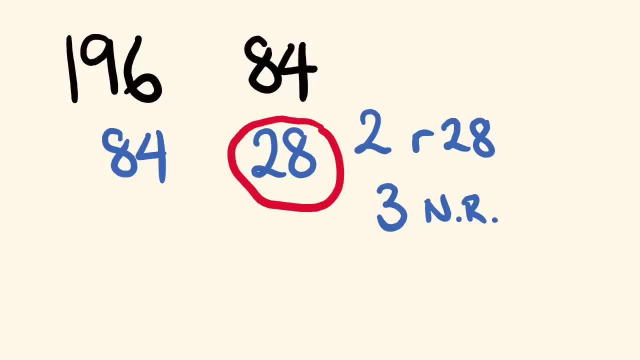 the greatest common factor. Okay, and it's this number that we divided into, Okay, the smaller of our two numbers here. Okay, so it's 28.. So did you get that? So, pretty much what we do for this method is we're going to be dividing the smaller number into the larger number of our two numbers. 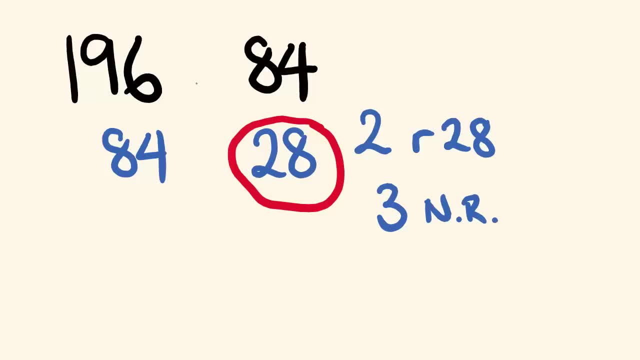 that we start with our two numbers. we're trying to find the greatest common factor of, And we're going to be moving any remainder onto this next stage, as well as the smallest one of them from the previous step, And we're going to continue this till we get no remainder. Once we get no, 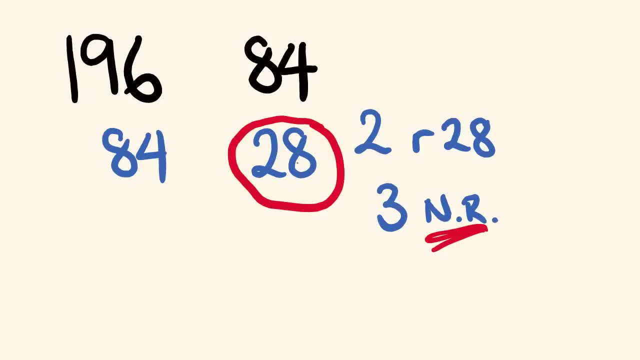 remainder, the number that we've divided into the other one. okay, the smallest of these two, that is our greatest common factor, or our highest common factor. Okay, so what about we have a look at a couple more examples? What about I give you an example with one that you're probably going to? 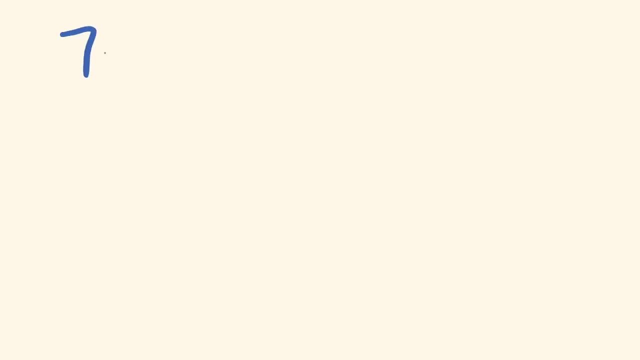 be able to look at straight away and work out the factors of, Say, we had 72, and 60. Now you may look at this straight away and go: okay, the highest common factor is that. and that's great if you can, But I'm just going to use it to show you this method. So, anyway, we're. 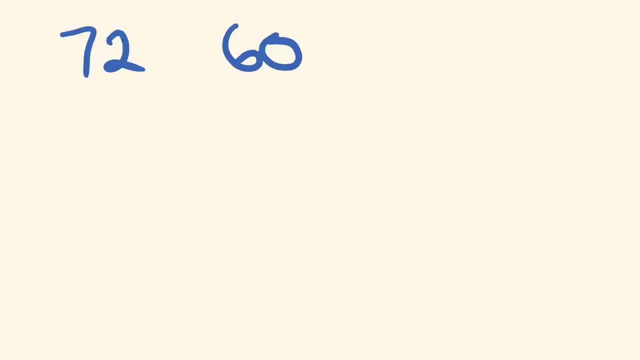 going to divide 60 into 72.. 60 goes into 72 one time, it goes in one time and it has a remainder of 12.. Okay, so this remainder, we're going to put down here And we're going to take the smallest. 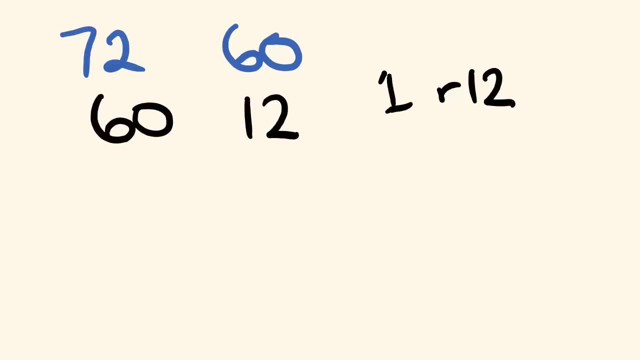 of these two numbers and we're going to use that for our next part. So now we're going to look at the 60 and 12.. How many times does 12 go into 60?? 12 goes into 60 five times, with no remainder. So 12 is our. 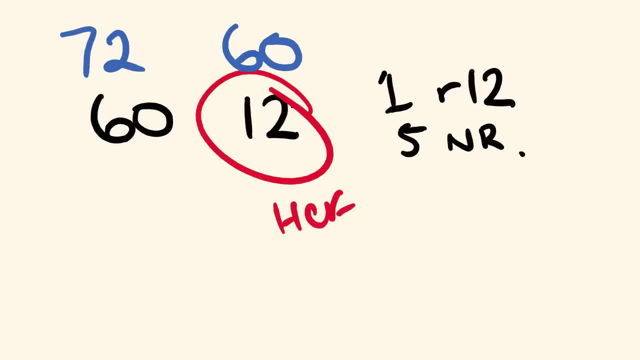 highest common factor. Yeah, did you get that method? Okay, what about we'll go through another one? Okay, what about I'll give you one? I'll go through one more together, then I'll give you guys another one. So we've got 148 and 48.. Okay, so we're looking. how many times does 48 go into 148? It. 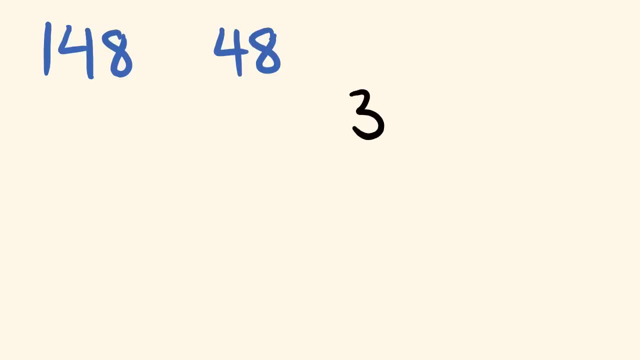 goes three times. Okay, 148 goes in three times and it has a remainder of four. Okay, so we're going to move this remainder here, this four here, and we're going to move the 48 here, the smaller of these two, down to here. Now we look at how many times four goes into 48.. Four goes into 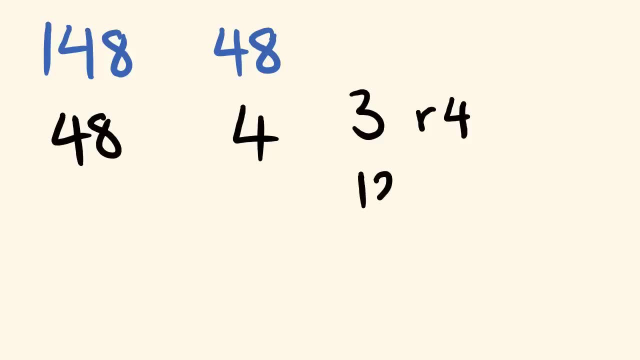 48, 12 times. Okay, it goes in 12 times and there is no remainder. So four is our highest common factor. Yeah, what about I'll give you a go doing this? Okay, so it's the remainders. we're. 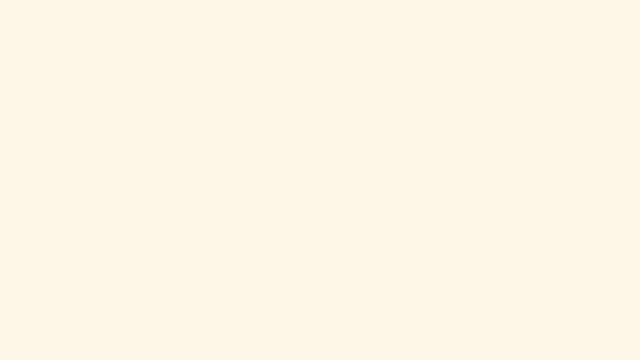 interested in. And this is a very, very old method. This is the Euclidean method of doing this. It's fairly old. Okay, what about you try this with 130 and 78. Then you might want to pause the video and do this. So hopefully you've done it, Hopefully you've given it a go, So we're 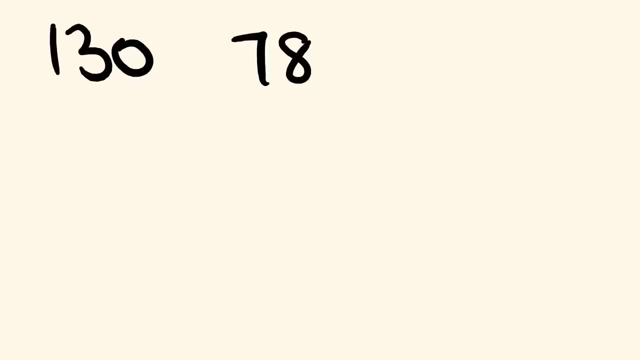 going to see how many times 78 goes into 130.. Okay, how many times is going to go in once and there is a remainder of 52. Okay, so I'm going to put this 52 here And I'm going to move the. 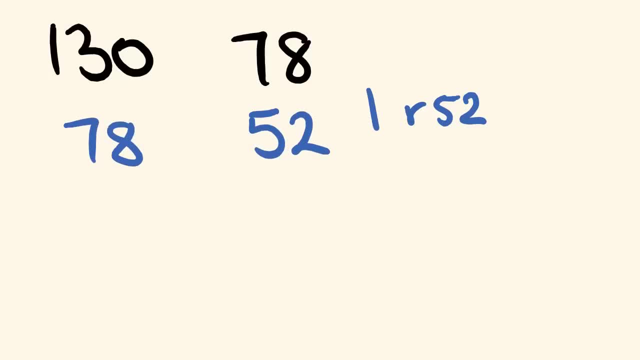 smaller of these two numbers of 78 down here. Okay, so now I see how many times 52 goes into 78. It goes in once. yeah, It goes in once with a remainder of 26.. Okay, so now I'm. 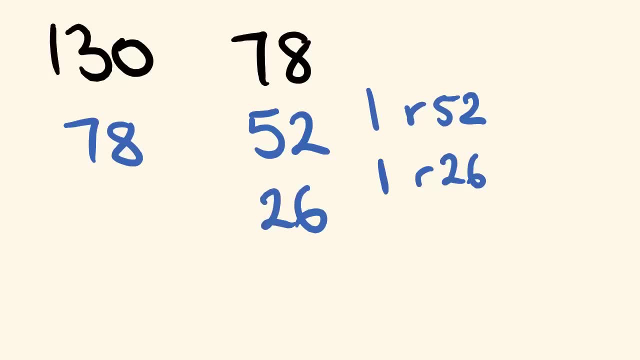 going to move this 26 down here. move the remainder here, move the smaller of these two numbers, the 52, down here as well. Okay, how many times does 26 go into 52?? It goes in two times No remainder. So our highest common factor is 26.. 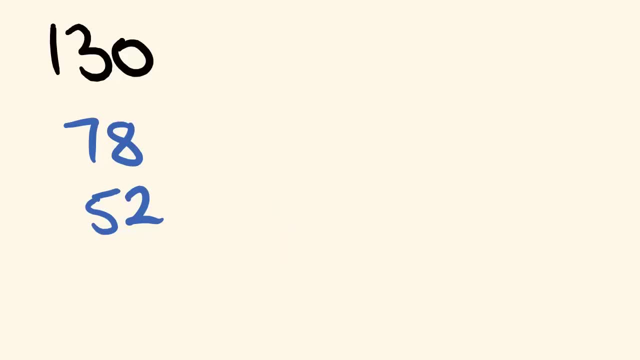 What about one last happy example for one of you guys? okay, And look, this does work for really, really big numbers. It's excellent. It's probably the best method for using with big numbers, Obviously small numbers. you can use your multiplication knowledge and that gets you. 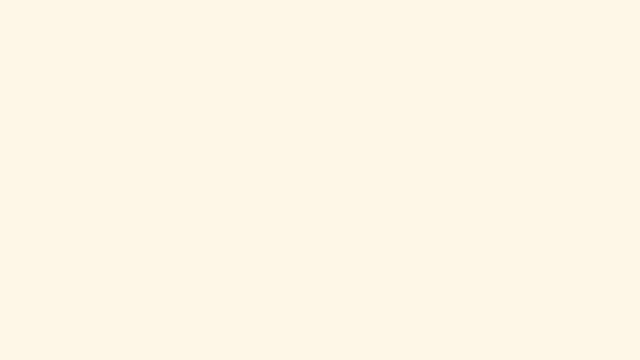 fairly far, But with bigger numbers, this is a really, really great method. Okay, so what about we give you this one? What about 585?? Okay, a really big number. Well, it's not really big, is it? But it's a big number: 585 and 105.. 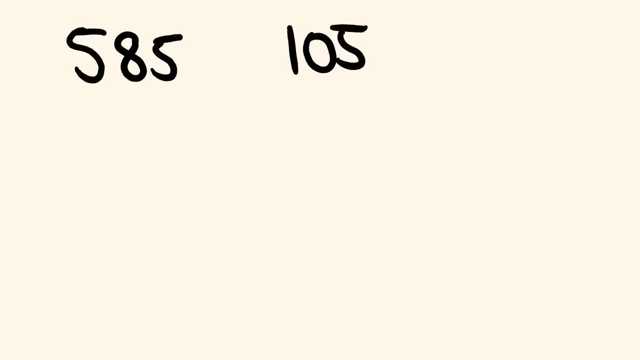 You get a look already and go, hey, five goes into that. But what would be the highest common factor of these two? So we start out. we'd see how many times 105 goes into 585.. It goes in five times. You can see that. Okay, so five times 105 is going to be 525.. There's a remainder of 60.. 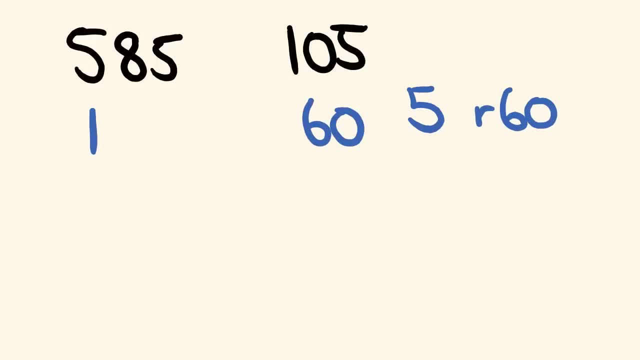 Okay, so I'll put the 60 here and I'll move this 105 down from here. Okay, all good. Yeah, okay, how many times does now 60 go into 105?? It goes in once, yeah, because two times would take it up to 120.. So it goes in once and it has a remainder of 45.. 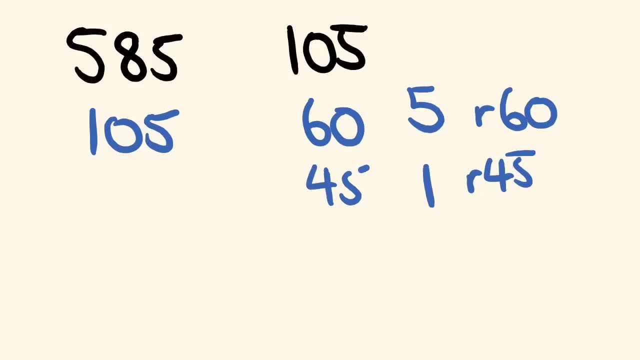 Okay, so we put the 45 here, put the 60 here. Hey look, you can see we're getting somewhere: 45 and 60.. Okay, numbers are getting smaller. How many times does 45 go into 60? Goes in once. 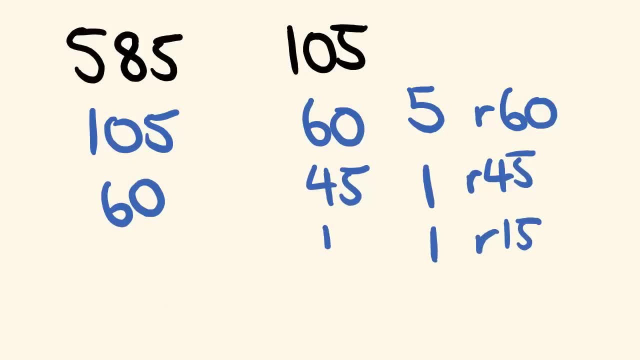 then there's 15 remainder. Okay, so put the 15 here: 45. I reckon you've just probably worked it out now what it is the highest common factor, because 15 goes into 45. It goes in three times. 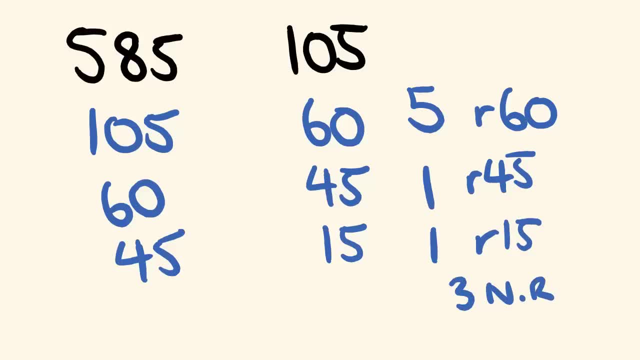 but it has no remainder. So our highest common factor- you might have guessed it is 15.. Anyway, hopefully you like this method. I'd like to give a big shout out. A few people will learn a bit to this. I made a video on factorization and how working at the highest common factor.